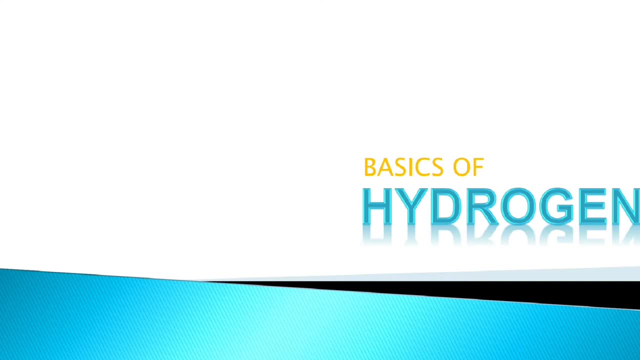 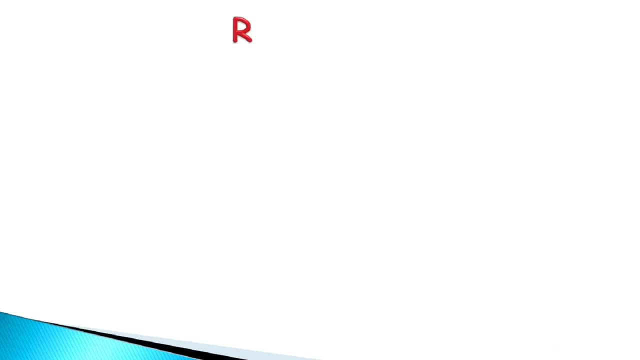 And what is its uses. So let's begin the first. what will be the road map which we are going to discuss in this lecture, is the first properties of hydrogen. Second is production properties, and why is the hydrogen unique? Then test for hydrogen and its uses of hydrogen. Now, when we are going to deal with the production of and the preparation of hydrogen, 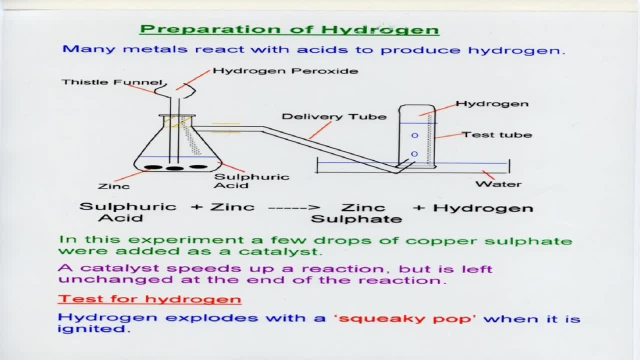 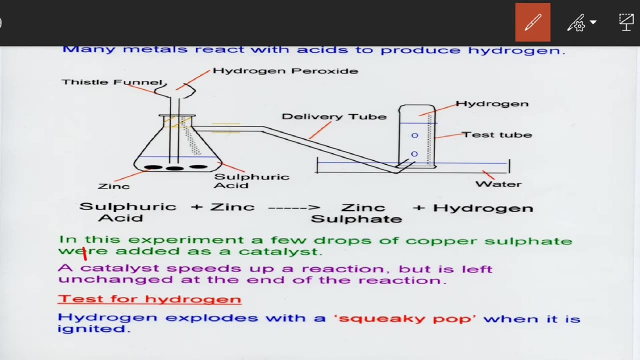 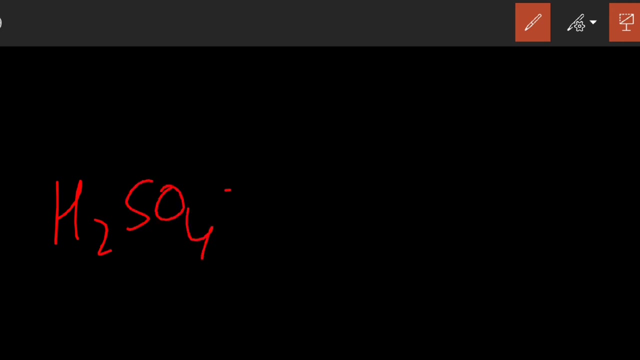 We see that the metals reacts with acid to produce a hydrogen. The metal reacts with acid to produce a hydrogen. Here is the example given over here: that this is the H2SO4 plus Zn means zinc gives hydrogen, ZnSO4 plus hydrogen. 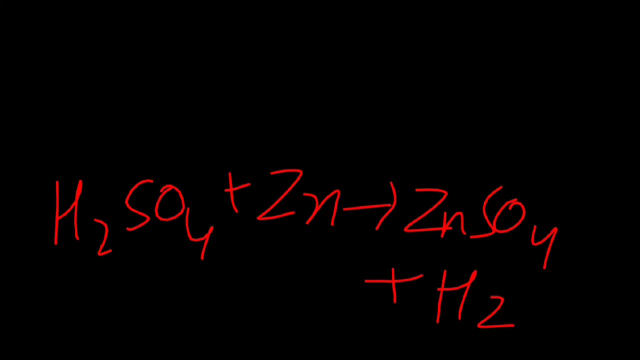 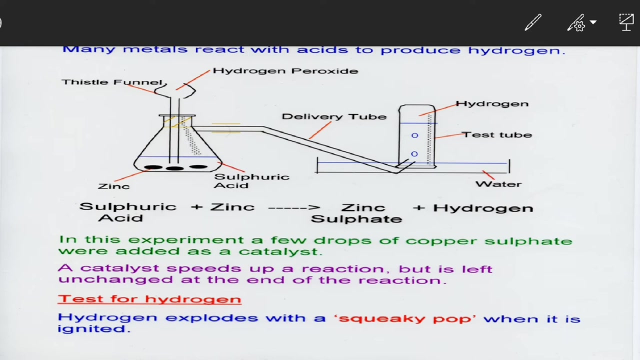 Okay, So this is the reaction I have told you. Basically, the production of hydrogen is that, as the reaction between a metal and acid produce hydrogen, We can place the reaction in a box that is connected to a delivery tube That will allow hydrogen to pass through it, Ending up in the water, through hydrogen will try to escape by bubbling up into the glass jar. 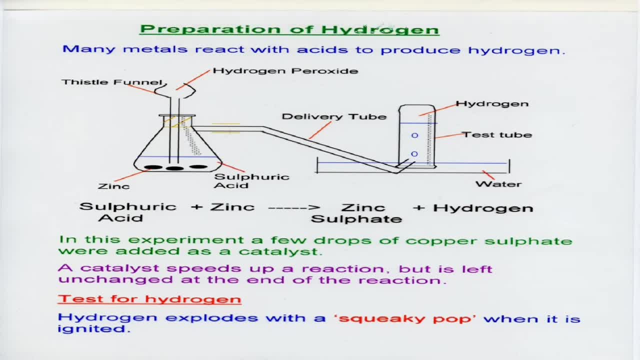 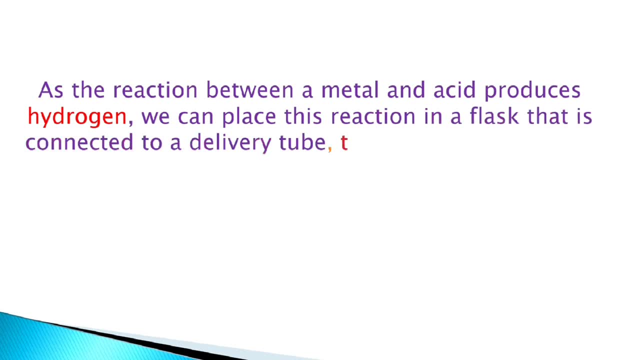 So and the taste of hydrogen we are going to discuss in the later part. Whatever I have said, this is on your screen. If you want to write the production of hydrogen, the procedure, the whole out map and the diagrammatically form, you can note it down. 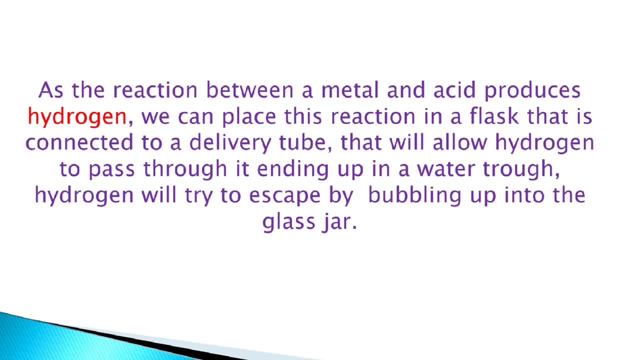 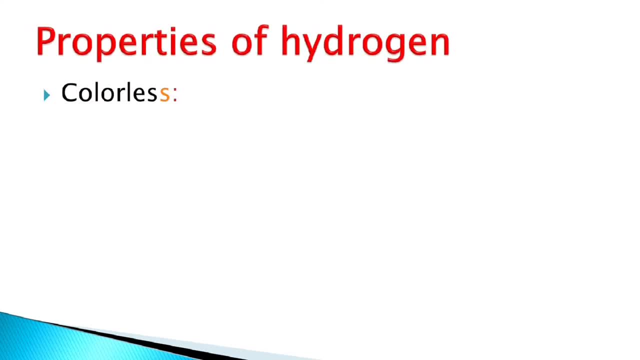 So I am going to Now discuss you the properties of hydrogen. So firstly, properties of hydrogen: It is colorless, Cannot be seen. It is odorless, Has no smell. It is tasteless, Doesn't have a taste. Gas found in a gas state. 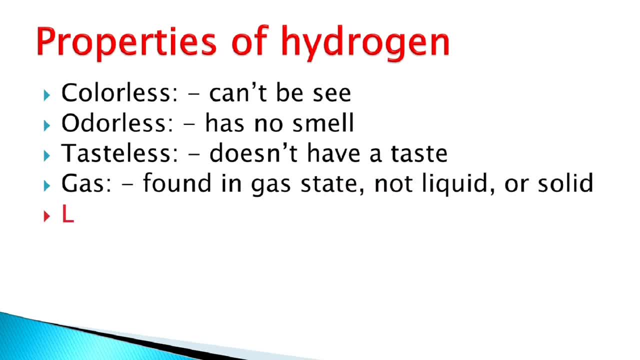 Not liquid, No, or solid. It is the lightest gas, Least density, Lighter than air, And it is accessible, Explosive. well, When it is reacted with oxygen, It gives water and a big amount of energy. It is exothermic reaction. 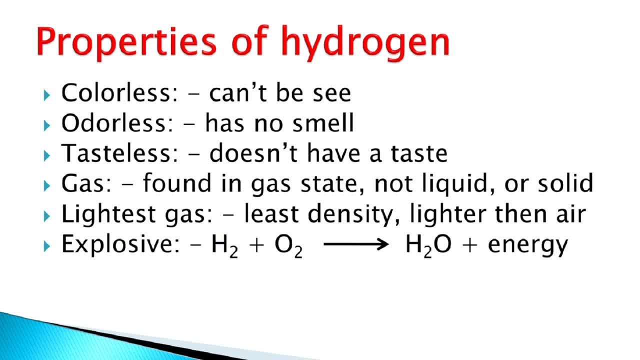 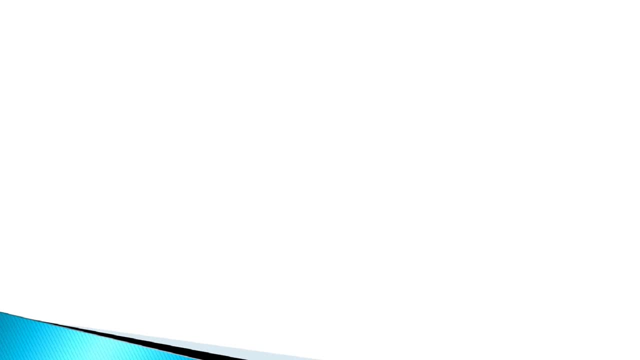 As you can see, It is explosive, So it react. Combine causes Explosion of H2 plus O2.. Now we are going to why the hydrogen is unique, If you are going to deal it, Why the hydrogen is unique, Hydrogen is known. 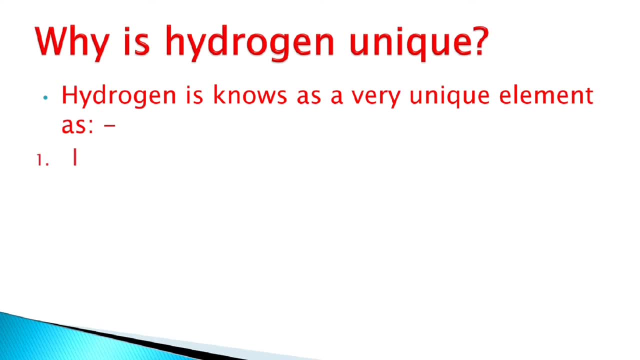 As very unique element, As it is a non metal In a group of one. Usually, elements in the group one Are metal. It tends to form More than one ion. It tends to form More than one ion. As you can see that. 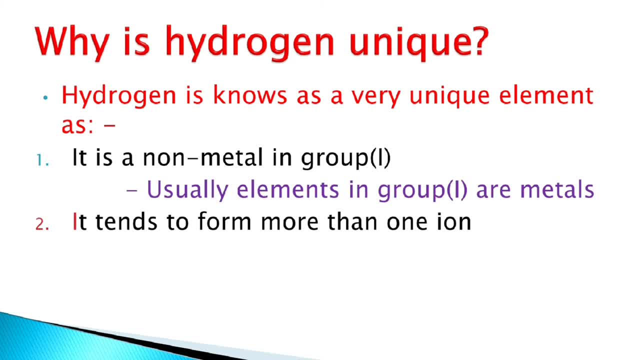 H1 plus hydrogen Mean, the proton H1 plus Is known as proton, And it is stable, And H1 minus Is known as hydride And it is unstable. It can exist in More than one ion form. 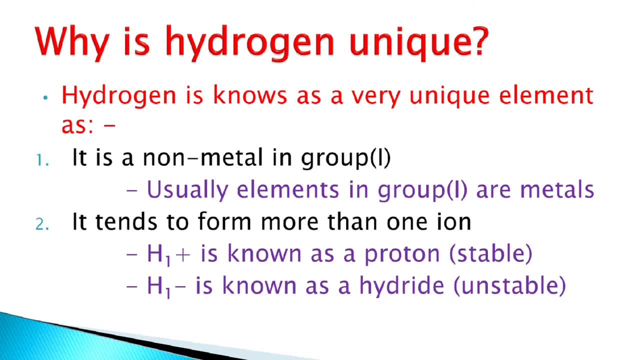 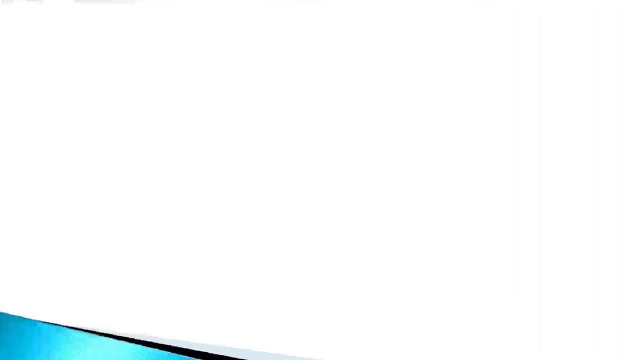 So this makes the Hydrogen unique. If you have studied very well Periodic table, It is the very unique doubt: Why Is hydrogen Is placed in Group one? We will discuss it later on. Firstly, we are going to take 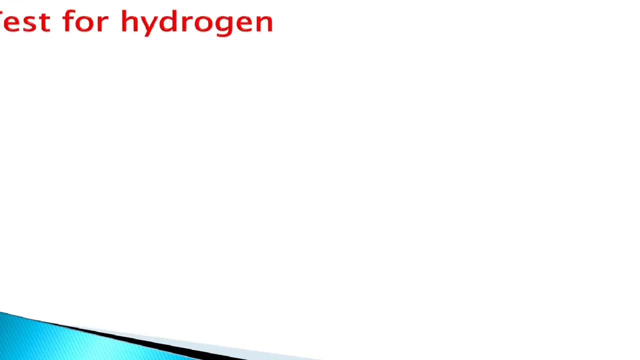 The test of hydrogen. For this I am going to tell you the very unique story That a boy and a teacher story. A boy forgets To label a container for two tubes, But he remembers that One of them has a hydrogen. 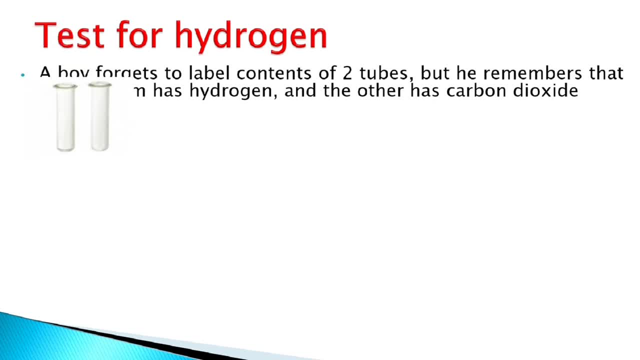 And other has a carbon dioxide, As this is the Test tube. Now the problem is here that The problem is here that both are odorless, Colorless, tasteless gases. So he asked the teacher: How do I test for a hydrogen? 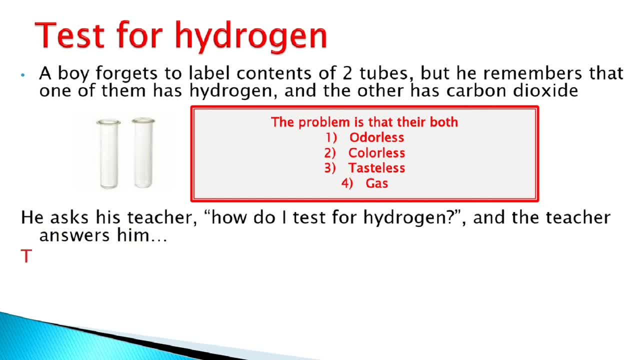 And the teacher answer him. Please do the test of this. That explodes. the gas To the lattice splint In the presence of oxygen. In the presence of oxygen It will be explode. You have seen in the properties of hydrogen. So he